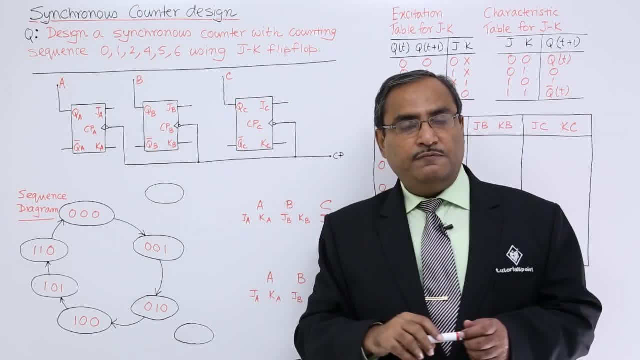 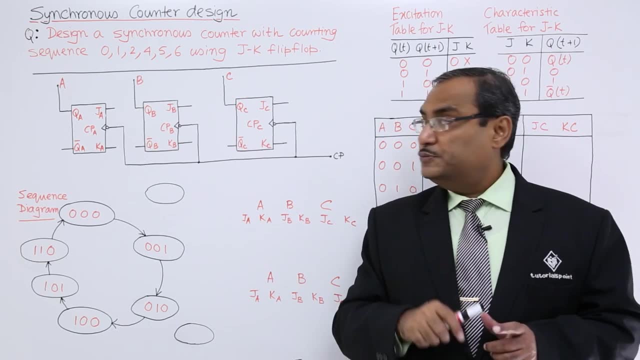 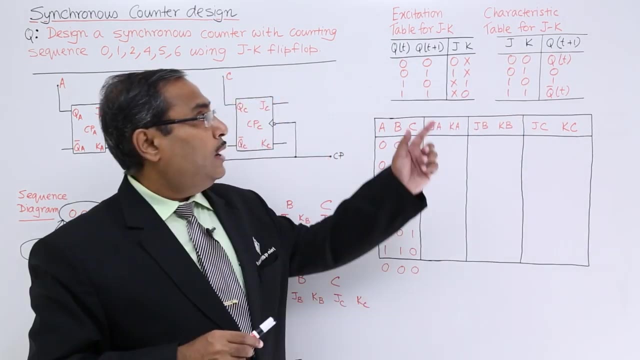 are supposed to get this G and K connections for the 3- 5th blocks. That means we are supposed to connect 6 such connections. So JK for 3- 5th blocks. So that is the thing, whatever we have done here, As we will be going to use the JK 5th blocks, so I have drawn the 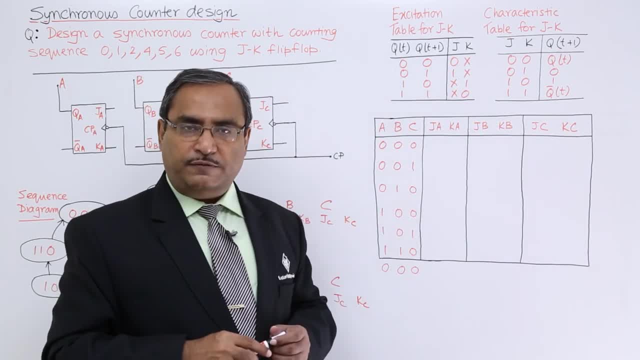 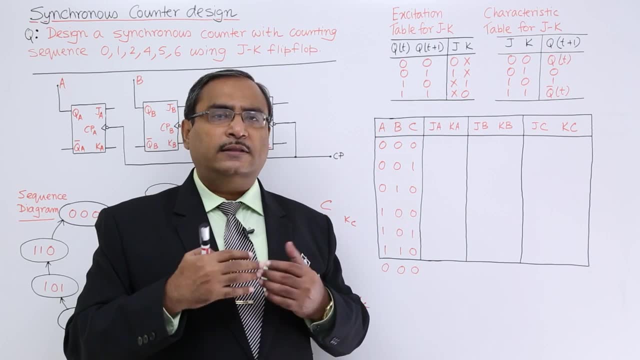 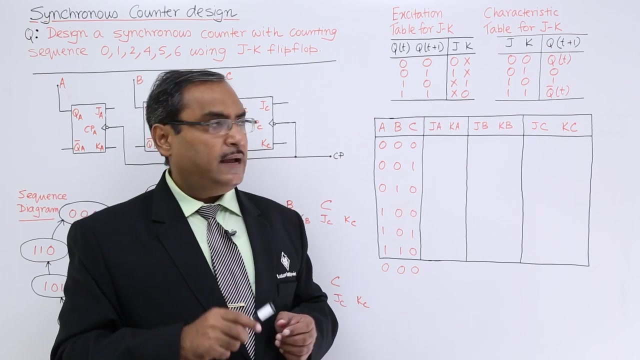 excitation table and also the characteristic table of the JK 5th block. So here we are having this: Qt and Qt plus 1.. Qt means the previous output or output at the tth instant of time And Qt plus 1 will be the current output. That means the output at t plus 1 instant of time. 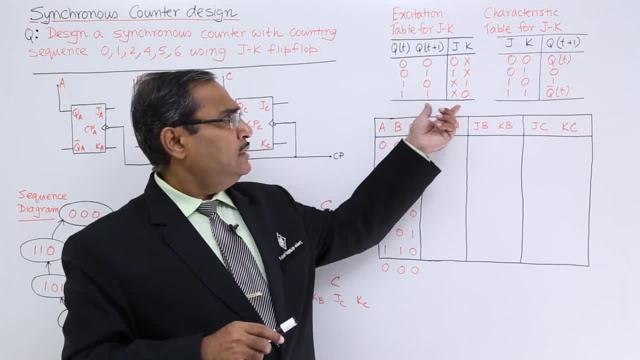 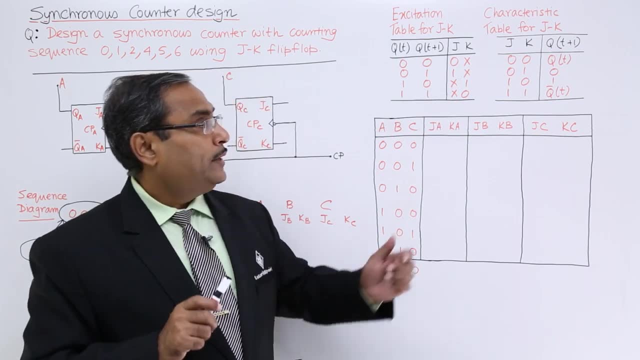 So here we are having this 0 0, 0, 1, 1 0, 1 1 combination, And here we are having the required G and K values, that is, 0 x 1, x, x 1 and x 0.. So here we are having the characteristic table. 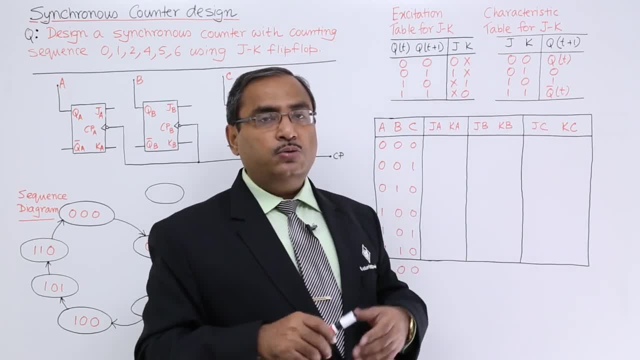 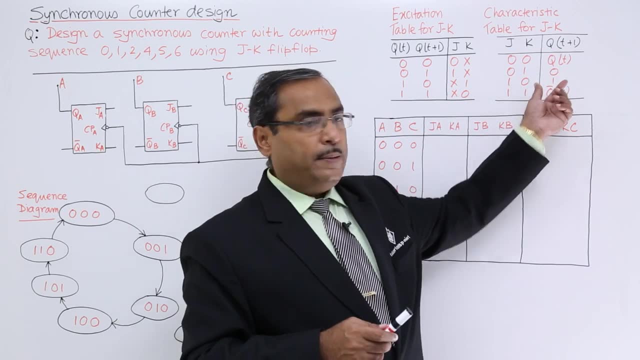 So here G and K will be the inputs and Qt plus 1 will be the output. In this case we are having Qt plus 1 and here we are having Qt 0, 1 and Q but T. In this way, this characteristic table. 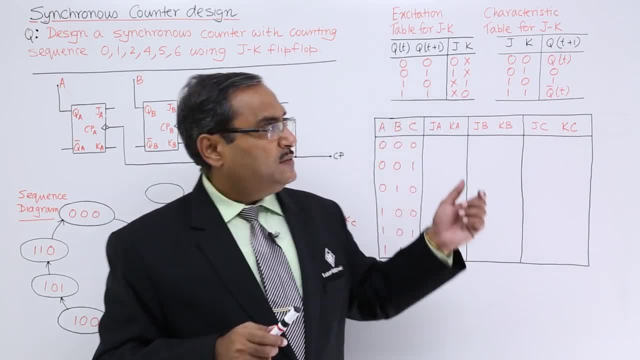 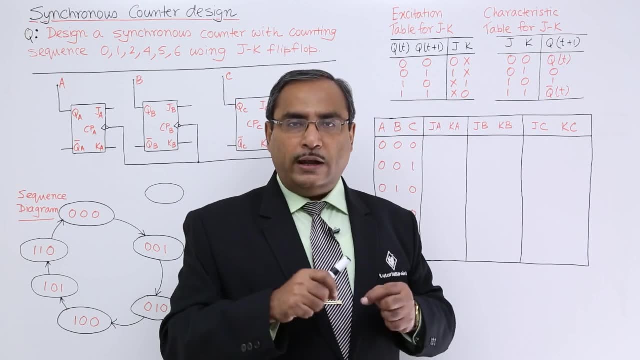 we have written. If we consider any other 5th block, then the respective excitation table and characteristic table you can keep on your answer sheet for your reference while doing the construction of the counter. So now, here we have written the sequence We have considered. 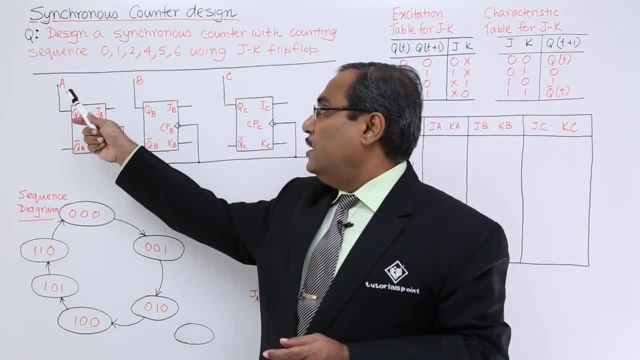 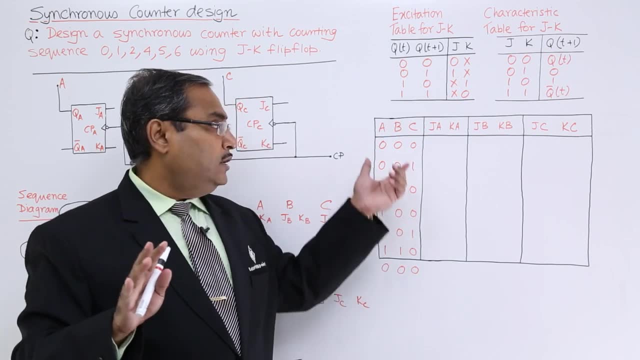 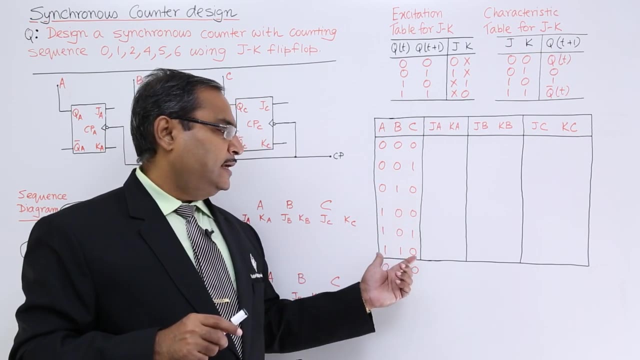 that the 5th blocks will have the outputs labeled with a, b and c, where a is the msb here here. So whatever the sequence, in synchronous counter design you are supposed to write them in this way, Here we are having the sequence like 0, 1, 2, 4, 6 and 5 and 6 here. So what? 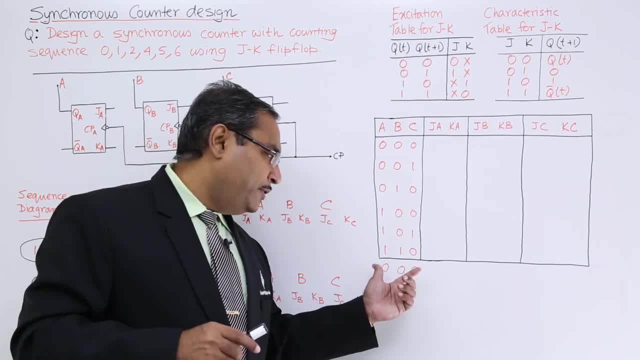 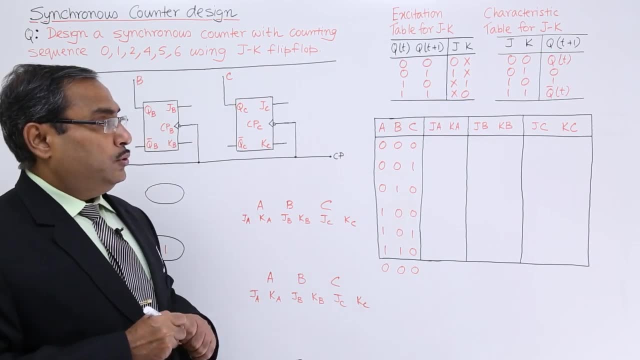 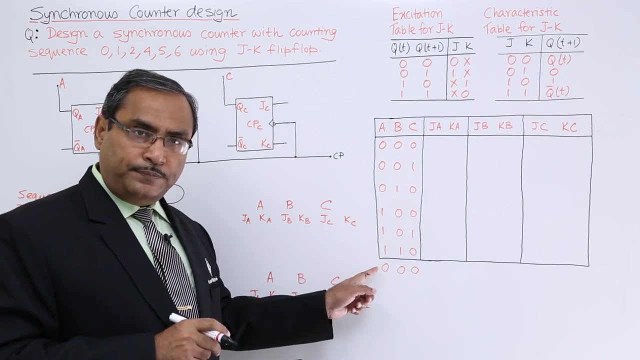 will be the next count after 6, then 0 will come back again. So I have written 0 outside of the table for my convenience. So now let me go for the counter design here. So we shall consider the excitation table for that. So we shall consider this a column and we shall fill up this. 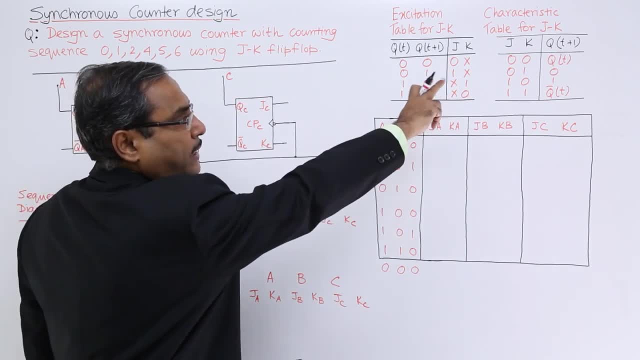 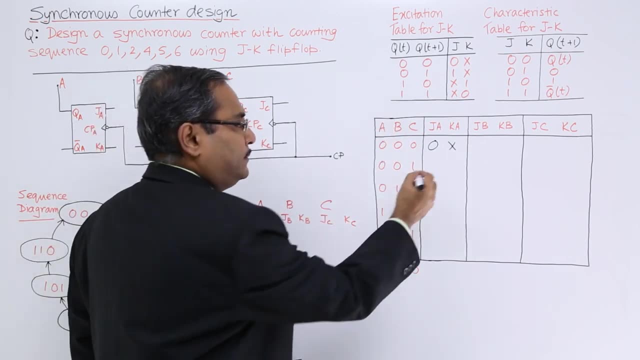 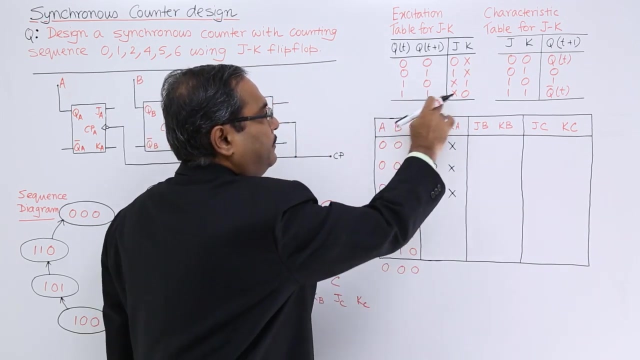 accordingly. So 0 to 0 transition we are having here, 0 to 0 transition is 0x. So I am writing here: 0x. 0 to 0 transition is 0x. 0 to 1 transition is 1x. 1 to 1 transition means x0.. 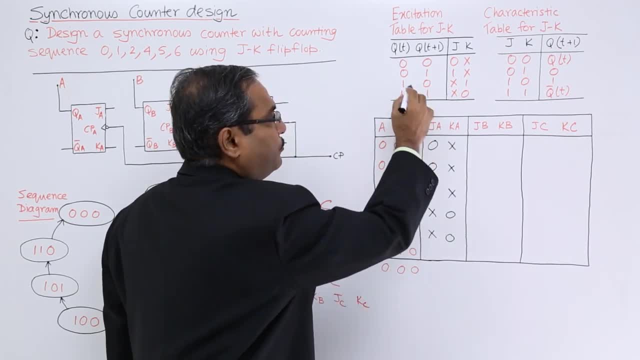 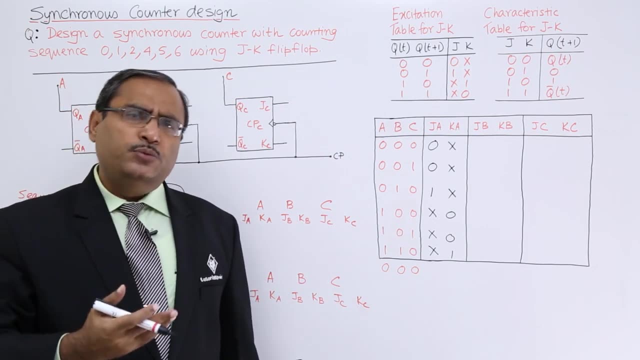 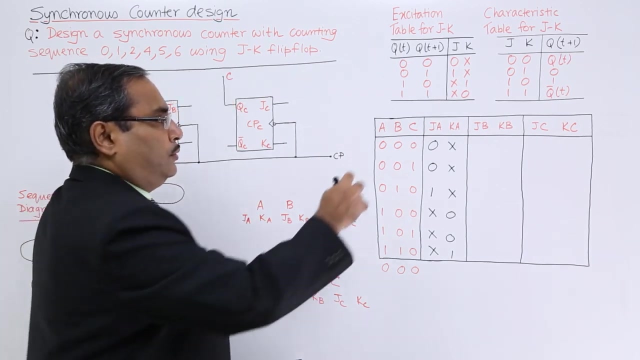 1 to 1 transition means x0 and 1 to 0 transition means x 1.. So in this way I have filled up j a and k a columns. So in this way we shall be filling up with j b and k b, j c and k c columns also. So for the 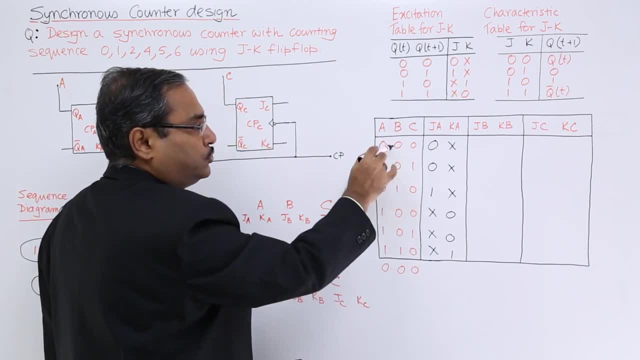 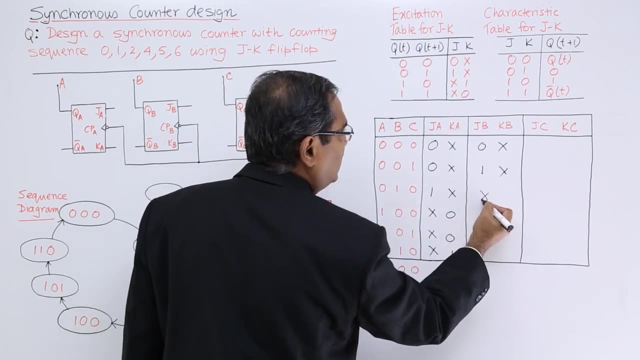 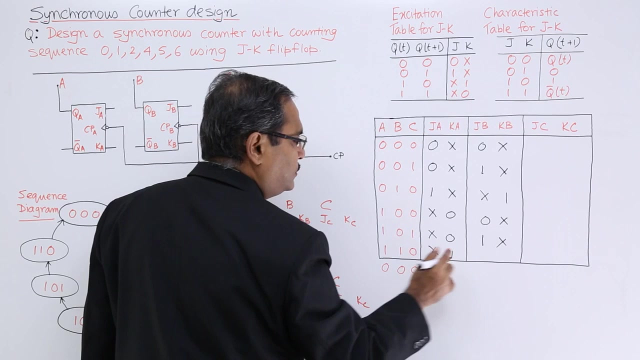 j, b, k, b. fill up. I shall be looking for the b column. So 0 to 0, that is 0 x 0 to 1, that is 1 x. 1 to 0, that is x. 1, 0 to 0, that is 0 x. 0 to 1, that is 1, x and 1 to 0, that is. 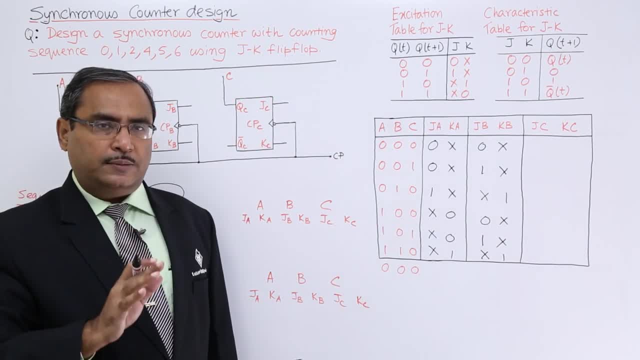 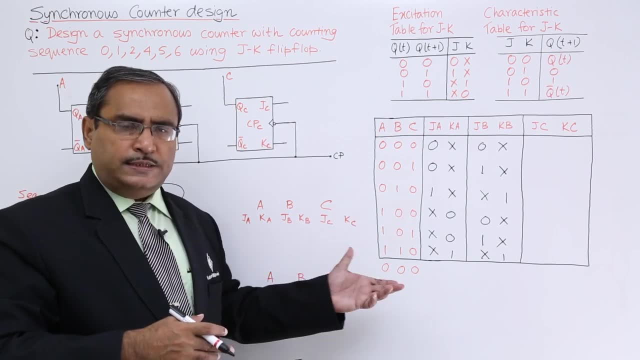 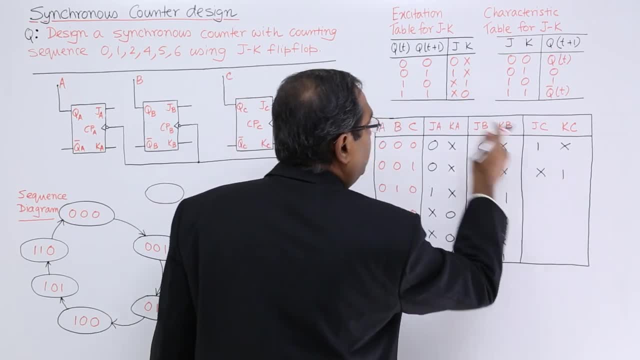 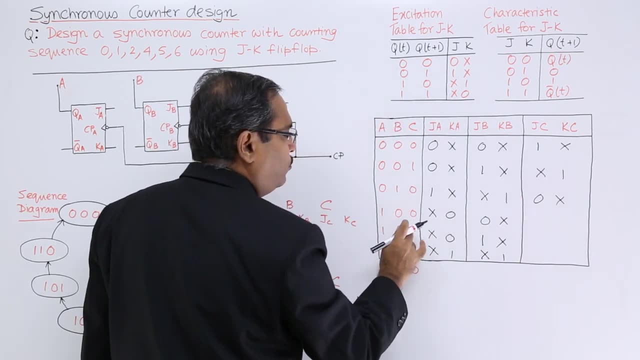 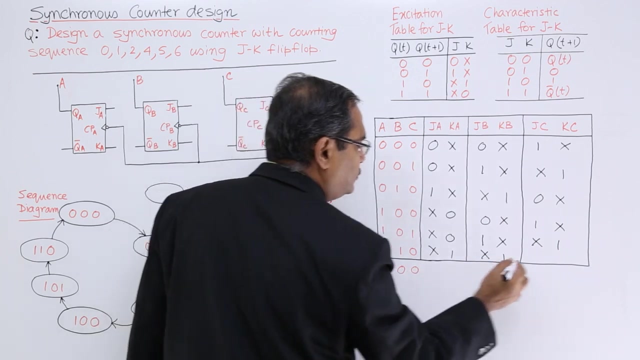 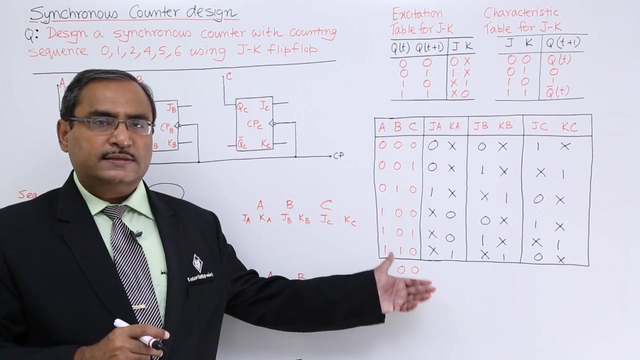 0 to 1, that is 0 x, and 1 to 0, that is 1 x. and here we are having this 0 to 0, that is 0 x. In this way we have done the fill up of all the 6 columns of j k. So now I shall. 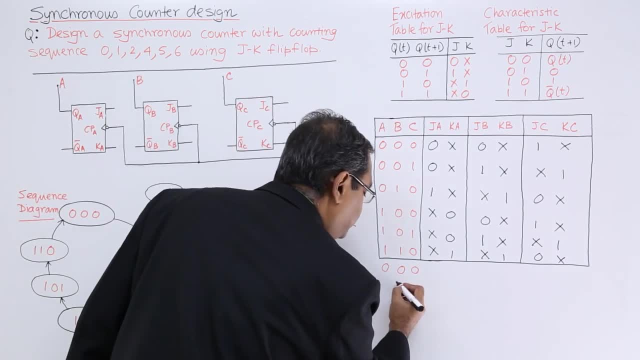 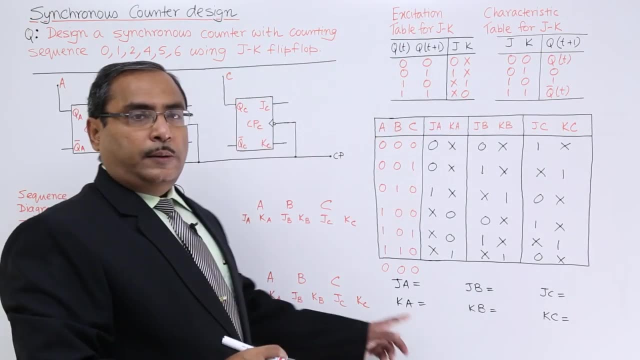 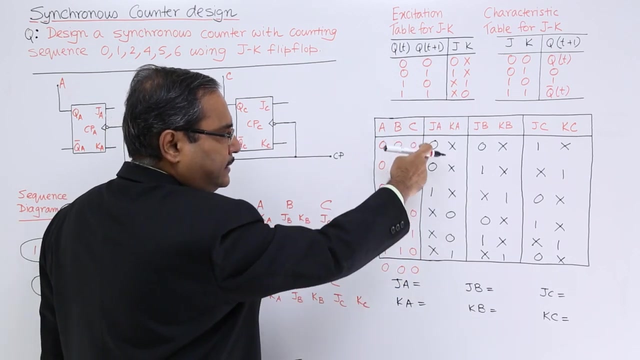 go for the respective summary. So I require to calculate j a, k. I have done it. Next I shall go for j a. So if you consider j a, you can easily find that j a is nothing but b. We require 0,, 0,, 1 and anything for. 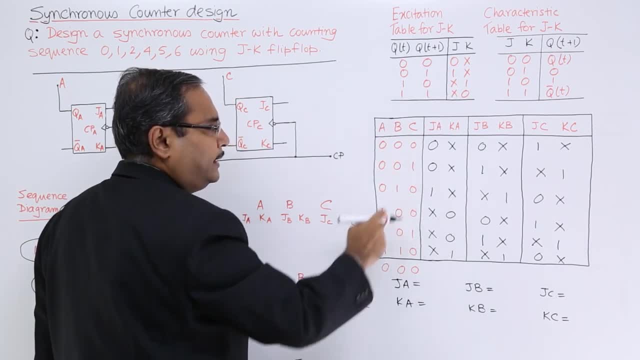 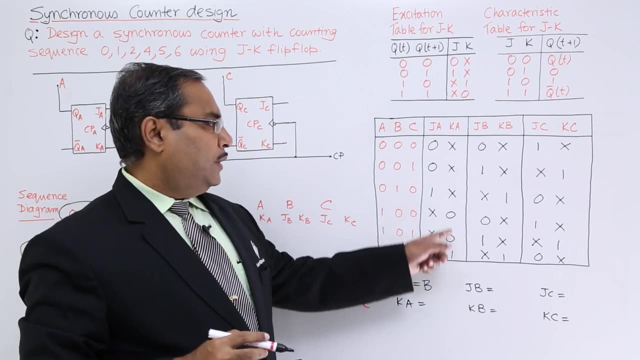 the rest So 0,, 0, 1. I am finding this one directly in b, So j a can easily be considered as b, So I am writing b here. So for this one, anything, anything, anything will be allowed. 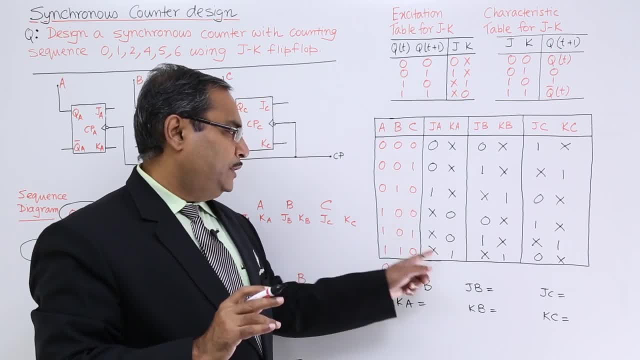 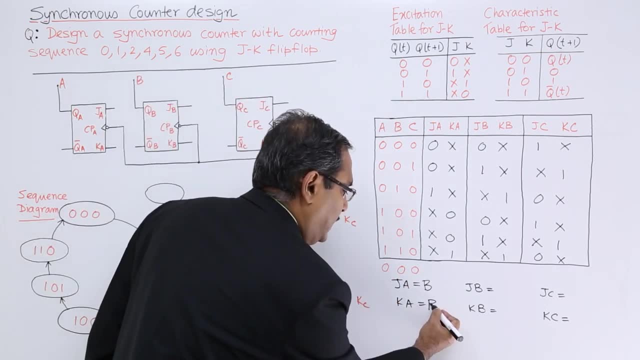 because x means do not care and 0, 0, 1 is should be there and that is matching with b. So that is why 0, 0, 1 is matching with b. So that is why for k a I am writing b. 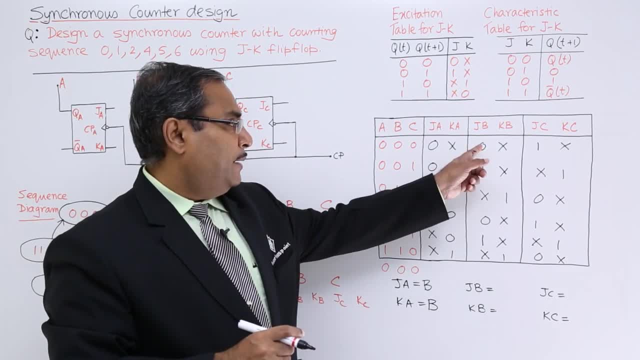 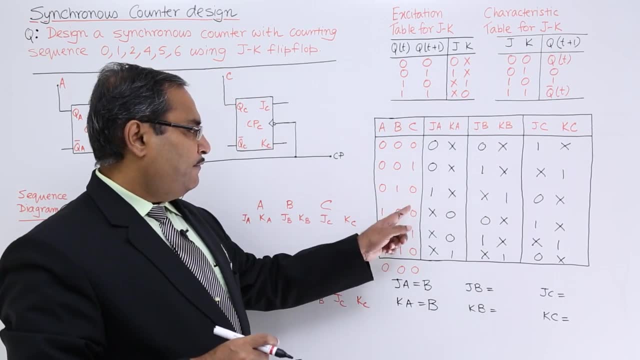 here Going for j b. in case of j b, I am. I am requiring 0, 1, anything and then 0, 1, anything, do not care, So 0, 1, I am finding 0, 1 here. 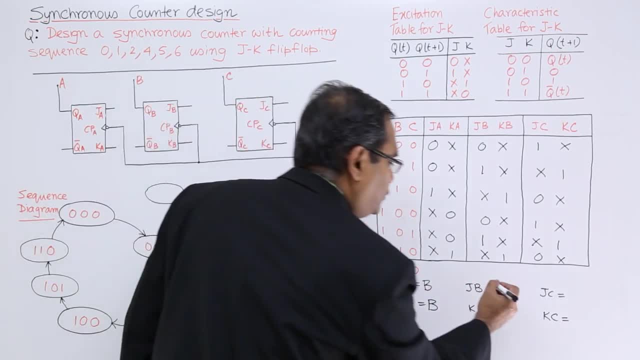 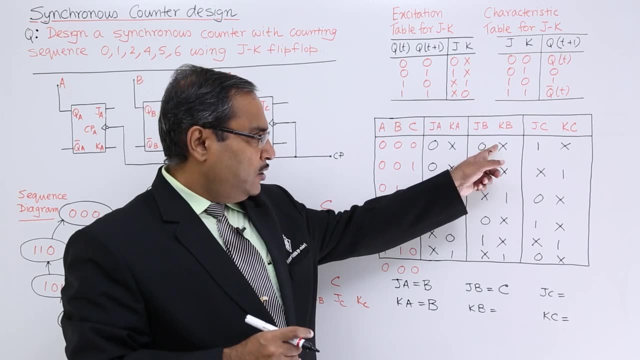 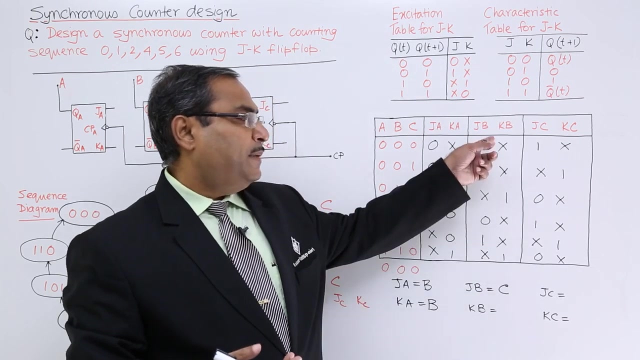 So j b is nothing but c. So j b is nothing but c. So I am writing c here. Now we shall go for this: k, b, k b. I am finding that throughout the column it is 1, because x can also be replaced by 0, can be replaced by 1.. So if we replace all the x by 1, so 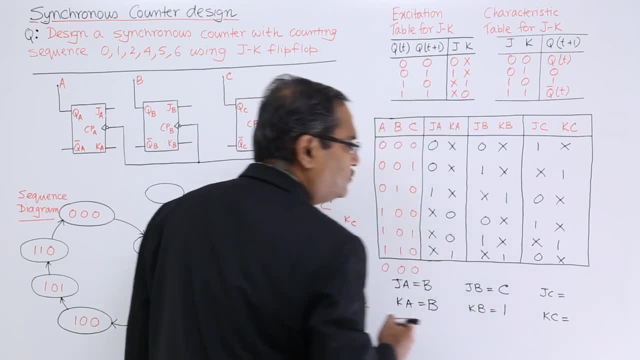 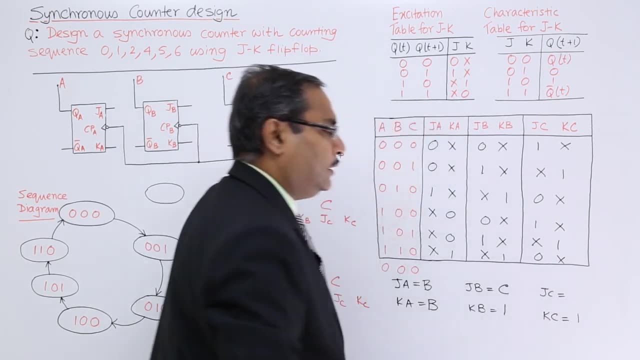 k b is 1 there, So I am going to write here k b as 1.. Similarly, if we consider this k c, k c is also 1.. So I shall be going for k c is equal to 1.. So I am remaining with. 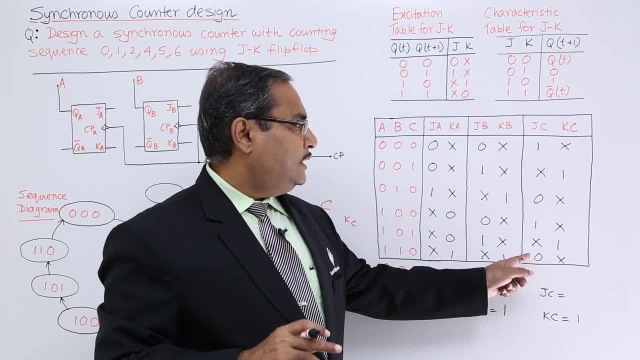 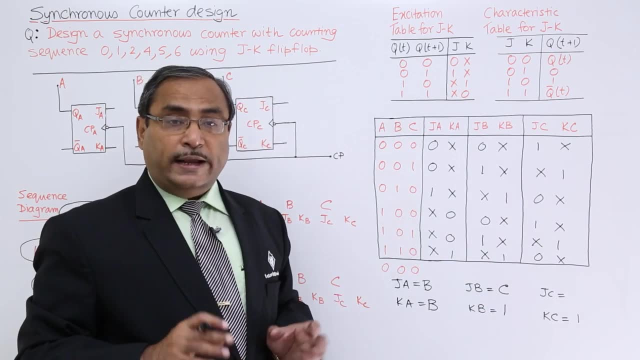 j c only. So if I, if I go for this j c, it is 1 x 0, 1 x 0.. I am not finding any parity here. So I think, for this j c, let me draw one Karnaugh map. So if you, if you having 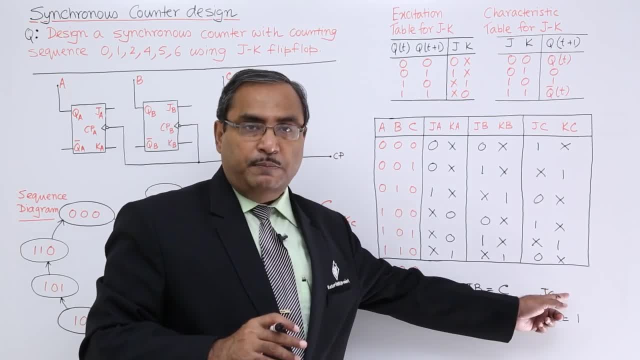 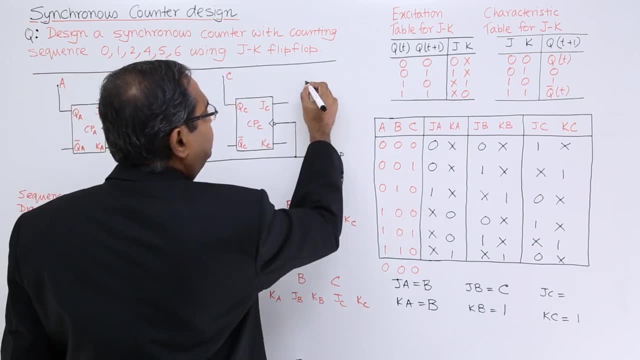 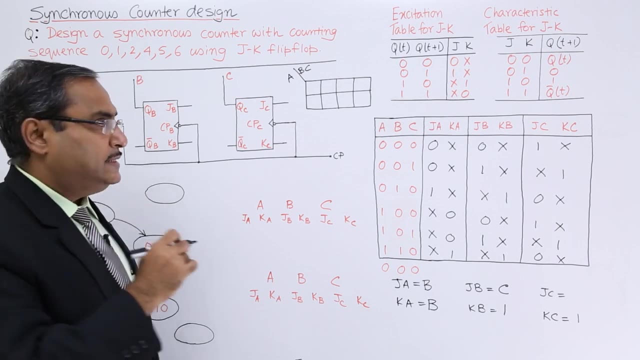 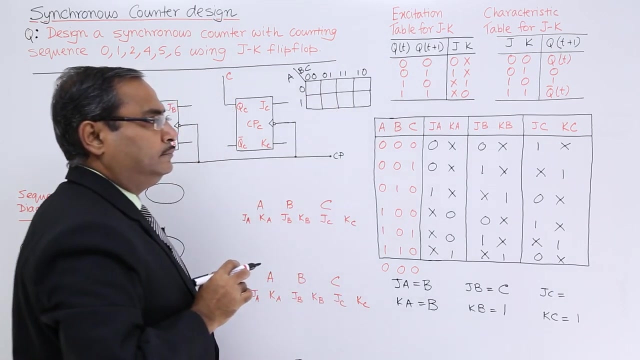 the way to find out the respective minimized equation for j c. you can easily get it, Otherwise Karnaugh map. Karnaugh map is always for us, So let me go for the Karnaugh map. So I have plotted here a and b, c. Now I shall plot here j, c. here I shall plot for. 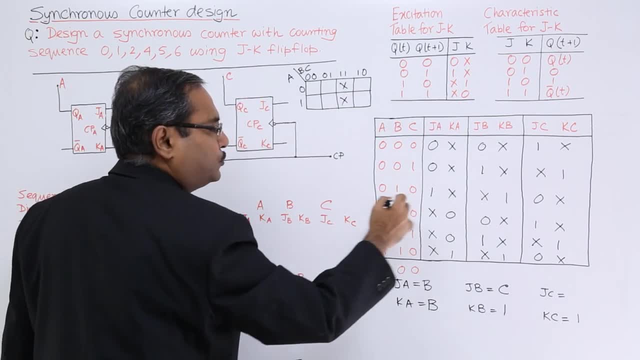 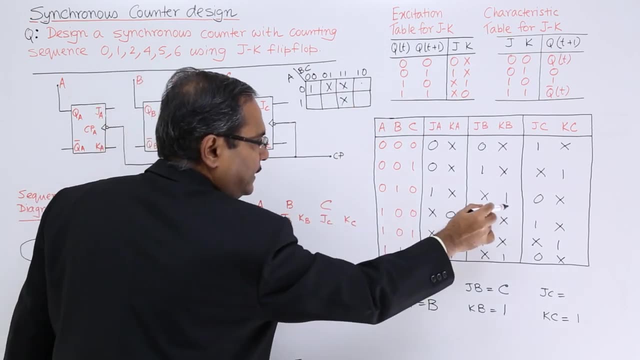 3 and for 7.. I do not know the required approach, So I put there x, So 1 x 0.. So 1 x 0, and here we are having 1 x 0.. So 1 x 0.. 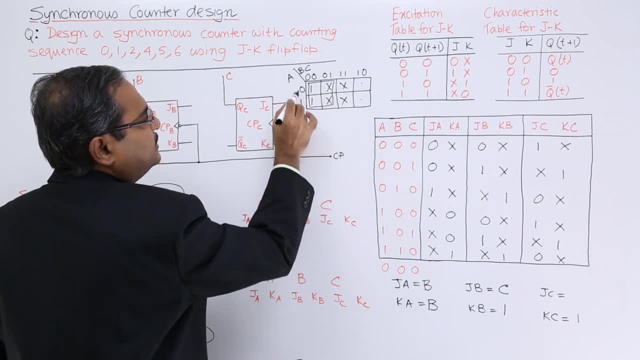 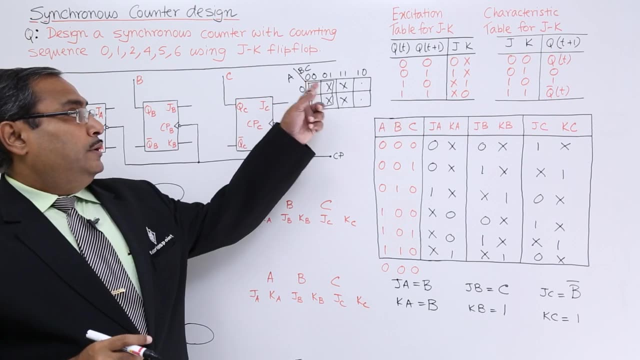 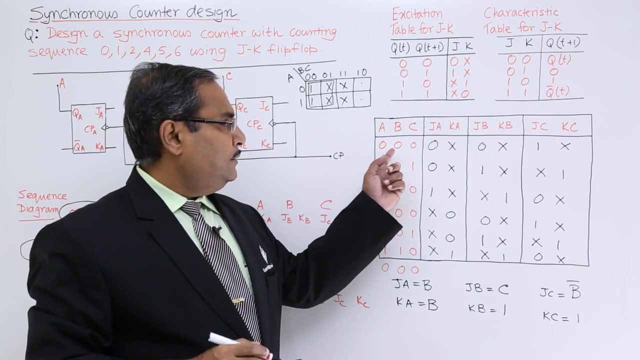 So if you do this covering- so I am finding a is not there, I will be finding b bar, I shall be finding b bar. So j c is equal to b bar. So here we are doing this kernel map and getting the minimized Boolean expression for j c. So you can also consider, you see. 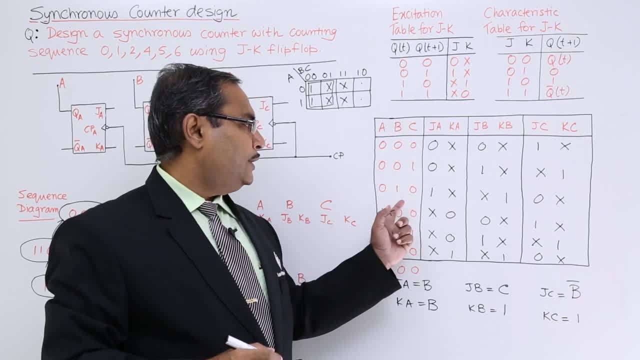 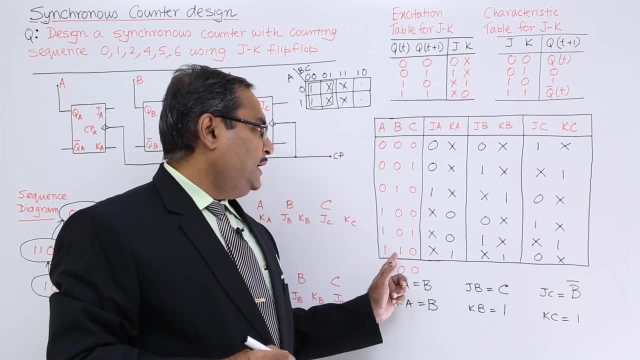 b is 0, j c is 1, b is 0,. it is: do not care, b is 1, j c is 0, b is 0,, j c is 1,. it is: do not care, and b is 1 and j c is 0. So it is obviously b bar. So also I have got. 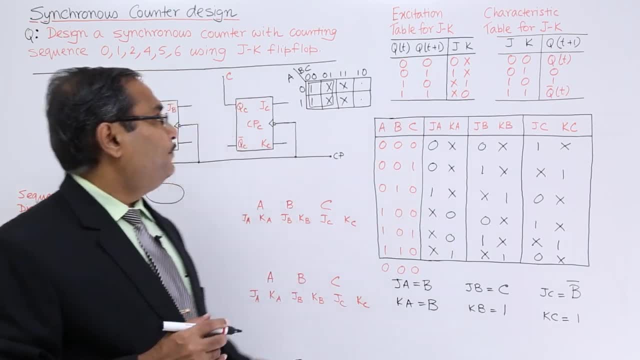 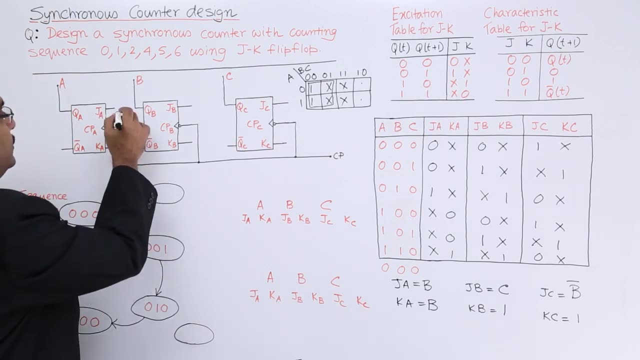 the indication from my kernel map also. So now let me go for the respective circuit design. So j k will be b and b. So I am just connecting this one to b and also this one. So whenever some connections are there, put such dots: So c and 1 here. so j b will be c and 1 here. 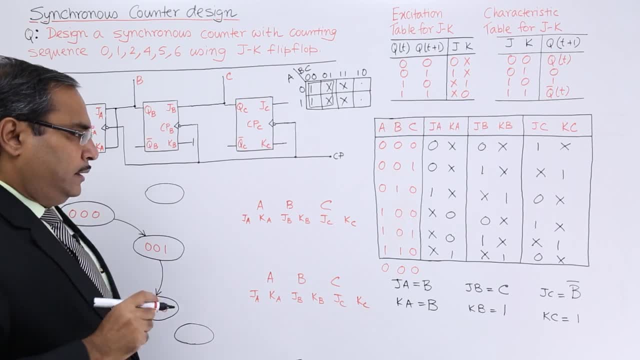 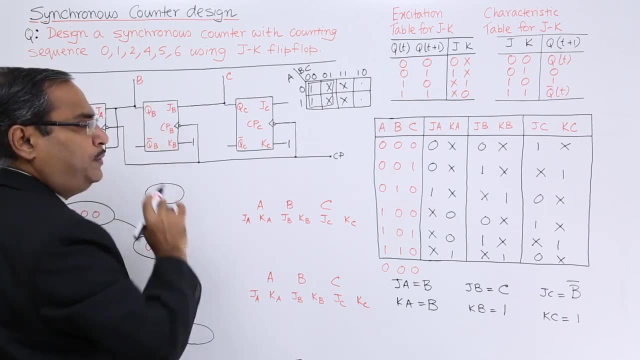 So j c will be b bar and k c will be 1.. So k c will be 1 and j c will be b bar. So q b denotes b. So obviously q b bar will be denoting b bar. So I am taking this b bar. 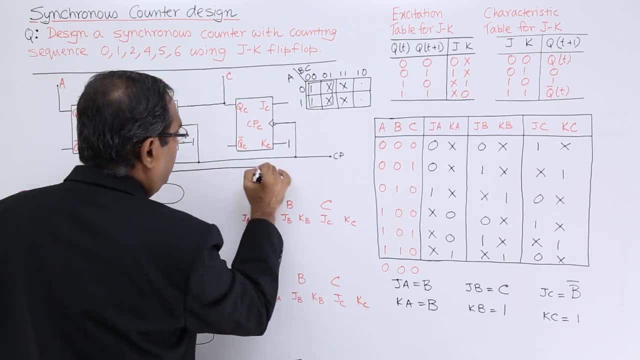 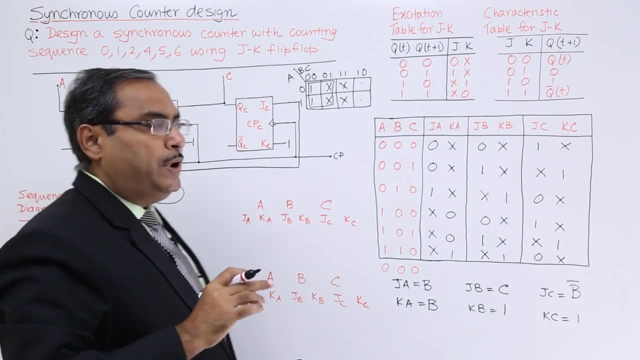 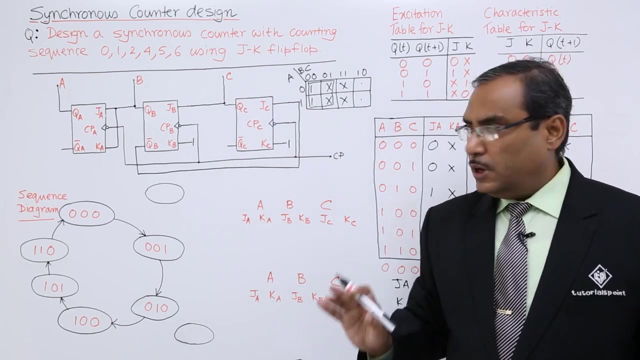 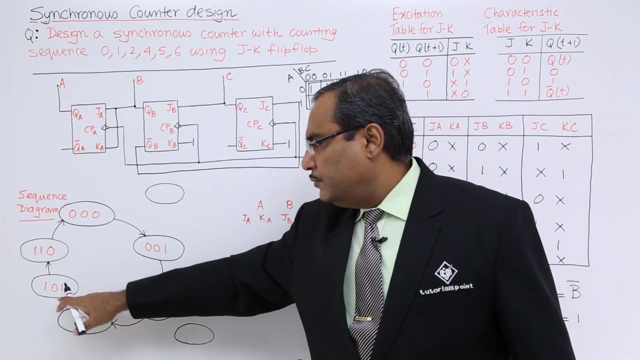 from here. So in this way I have completed my circuit diagram. So that is the circuit diagram I have drawn for one synchronous counter. So now this is my sequence diagram, So from 0,, then 1,, then 2,, then 4,, then 5,, then 6,, then 0 again. So I want to know that, if I 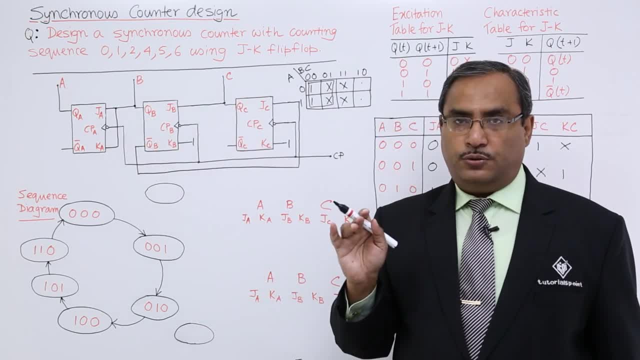 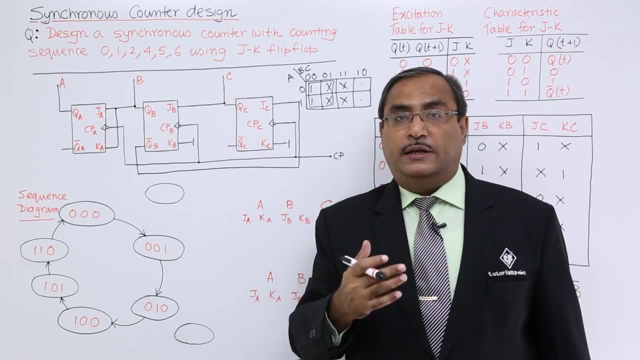 can make all the outputs 0 0, 0, making all the respective hip-clops reset. then if I make the next clock pulse, if I give the next clock pulse, then what will be the next output? The next output will be 0 0, 1.. So this is my sequence diagram. So this is my sequence. 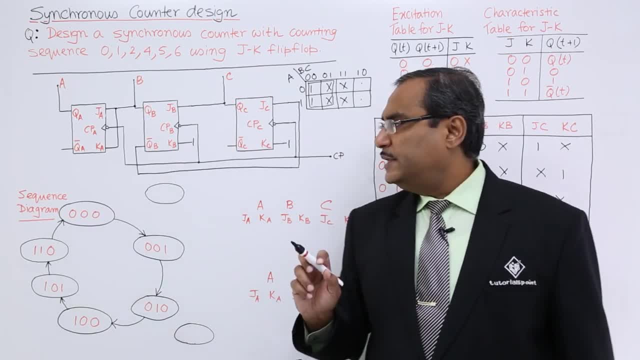 diagram. So now this is my sequence diagram. So from 0 then 1, then 2,, then 4, then 5, then 6, then 0, 1.. In this way we can easily get the sequence diagram. But what about those two? 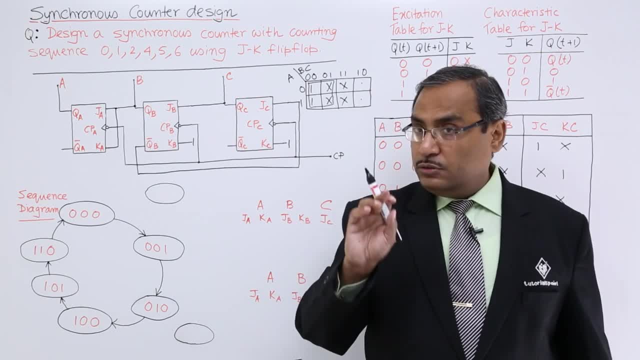 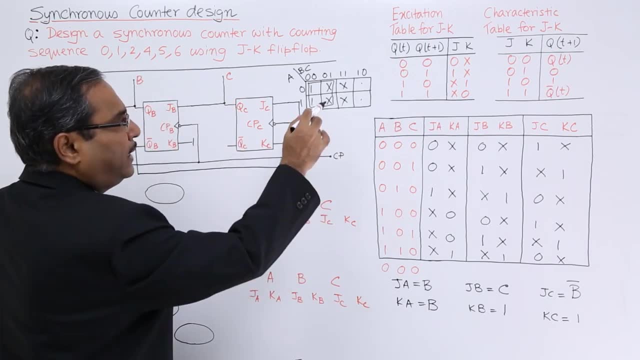 missing sequence. So one is our 3 and another one is our 7. So now let me work on them. So I am going for here, So I am going to calculate, because you see the 7 is missing. 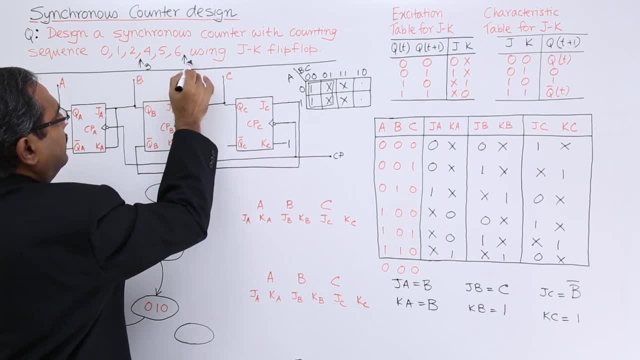 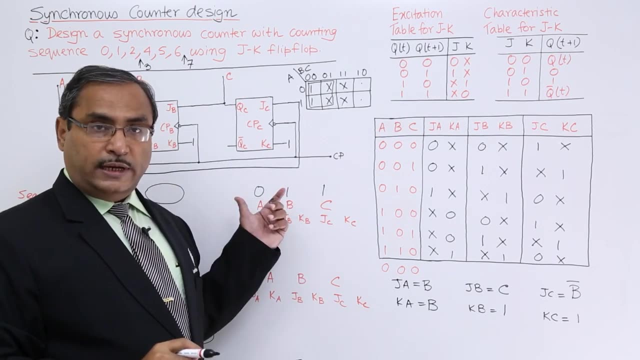 Here the 7 is missing and here this 3 is missing. So let me work for them. So I am considering 3 at first. So 3 means 0,, 1,, 1. So that is the 3. So I am going to consider 3. So 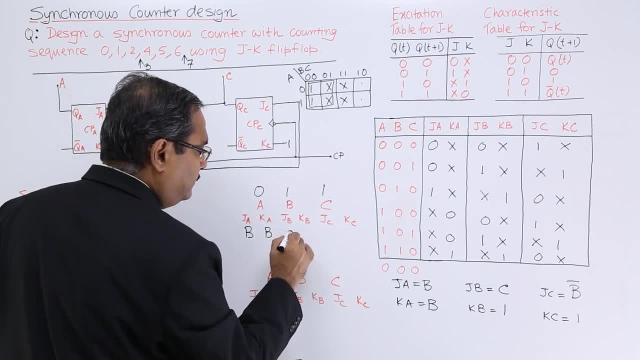 here the 3 at first. So I have already considered complex- which are playing out. How many of them has been these solutions before this particular 4? all these 2 is missing, but I am not forgetting the 3 after all this, So I work on all the new ones. This is how. 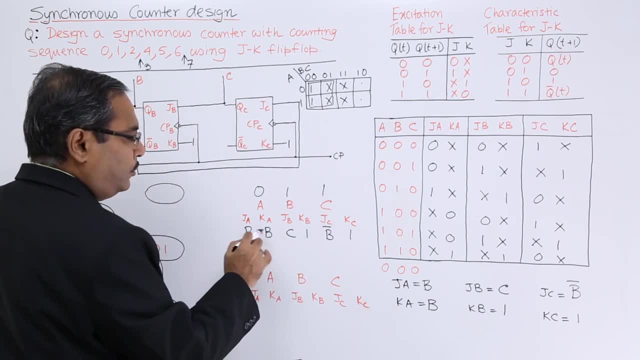 I говорить this problem. ok, So now in 3 container we are going to get 3 values. so 3 here, 0 and 0 here between the 3.. Now what do we have when they are 1, 1?? 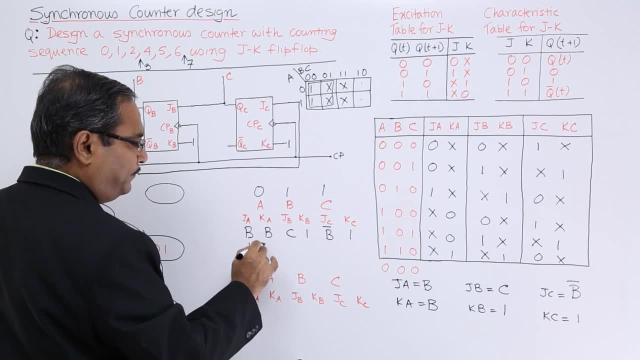 3 here, 0 here, 0 here, 1,, 1, and 이제 I am going to write over here that 3 is missing. Many of them are missing, but that is also working too. What we have to do, that is. 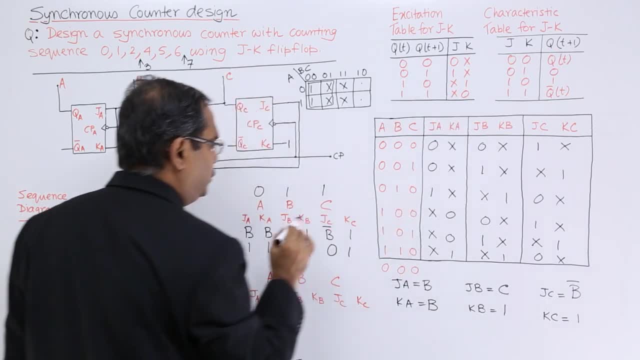 we have to take again in the same order For this curve. we have then 0.5, which means 0.5.. So what about those 2 values then? how many of them are armor sum If I take these values? 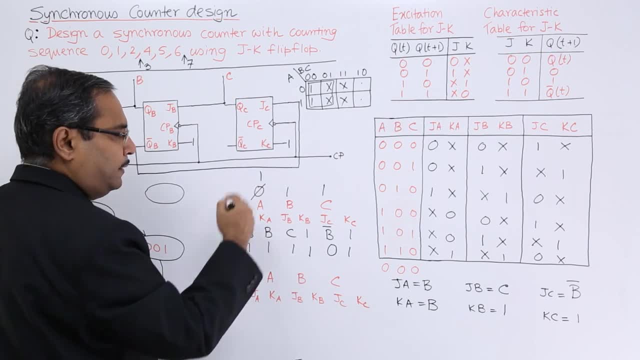 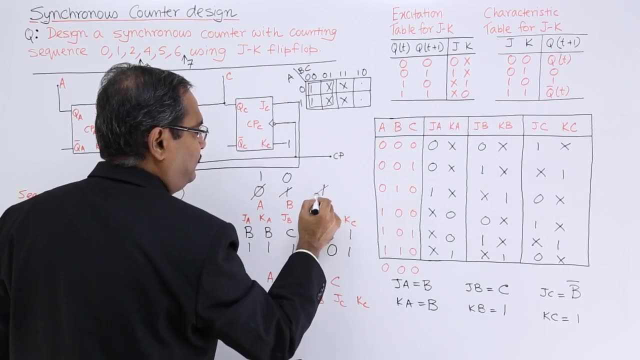 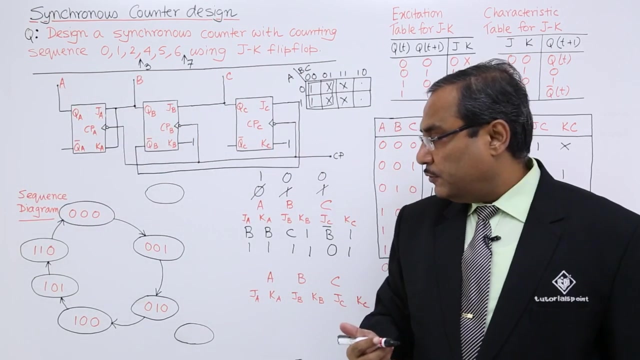 So 0 will be converted, will be replaced by its complement value: 1: 1, puberty: 0: 1, 0. 1 means 0. So from 3, I will be going for 4, from 3, I shall be going for 4.. So in this, 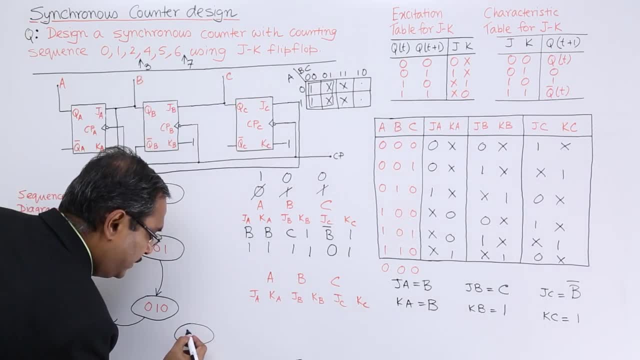 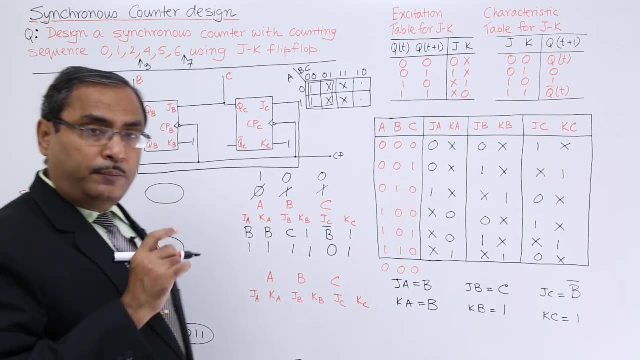 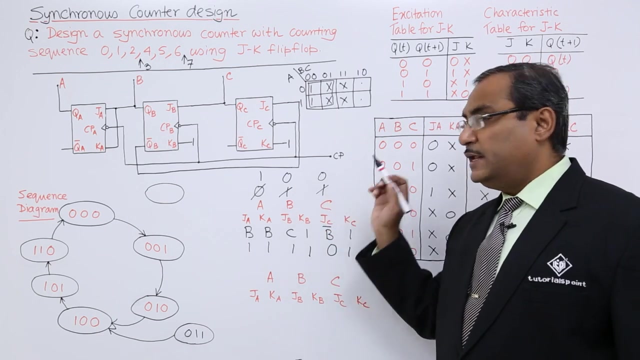 way I can. I can easily write the respective sequence, that is from 3.. So I have completed this one. So from 3, if I give the clock pulse, that means, if I make this flip-flop reset, this flip-flop set, this flip-flop set, and if I give the clock pulse, the next output. 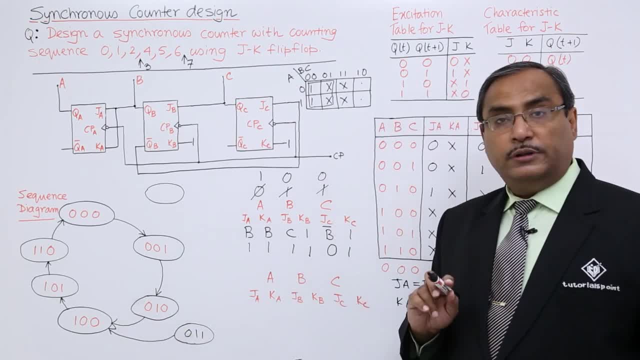 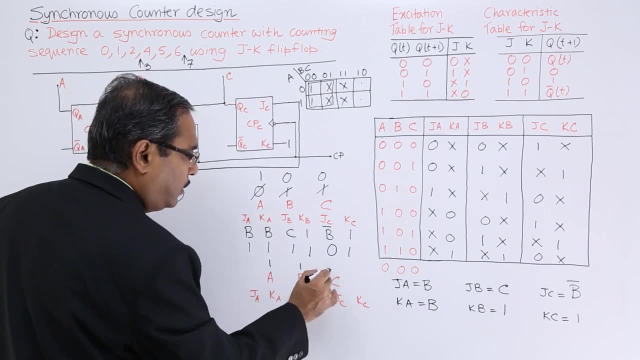 will be 1 0, 0.. So that is why I have drawn this one. I have drawn this one. Now the next one here. the sequence 7 is missing. So for the 7, I am writing here: 1 1, 1,. I am. 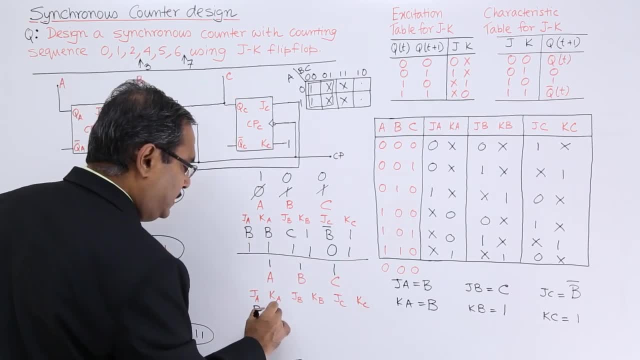 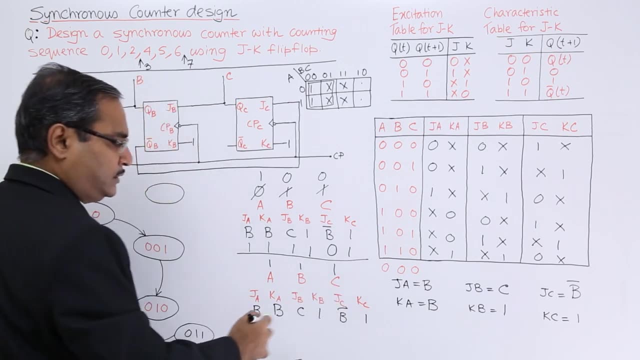 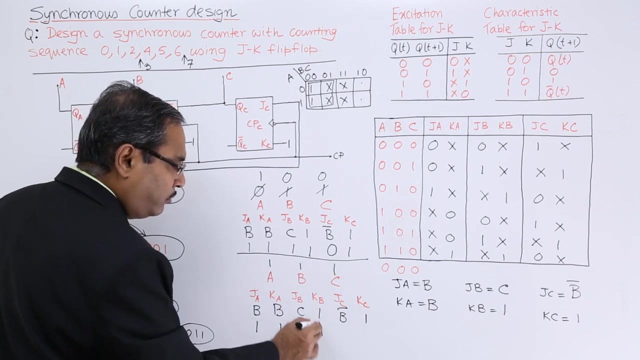 writing here 1, 1, 1, and this is my V b, c, 1 applicable. So according to the formula functions, Boolean functions. I am getting this. So now b is 1.. So I am putting 1, 1 here. c is 1, I am putting 1 and this is 1 already. b is 1.. So. 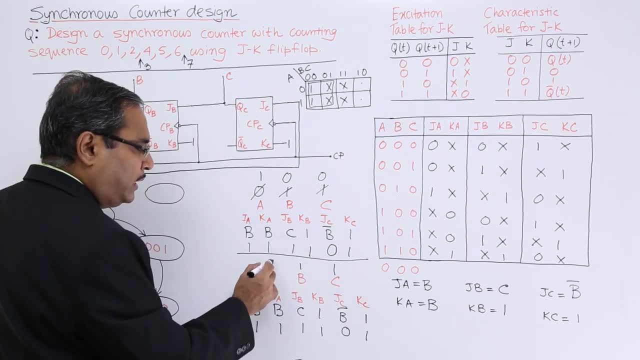 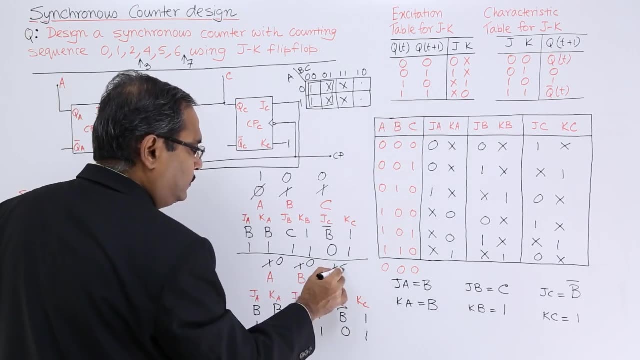 b bar will be 0 and this is 1.. So for 1: 1 output will be complemented for 1: 1 output will be complemented for 0: 1 output will be 0.. So that means from 7, that is 1: 1, 1. 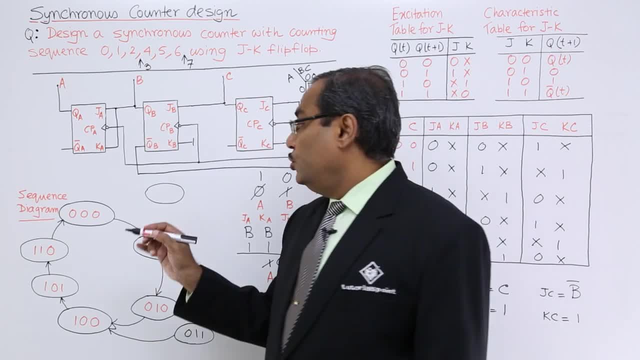 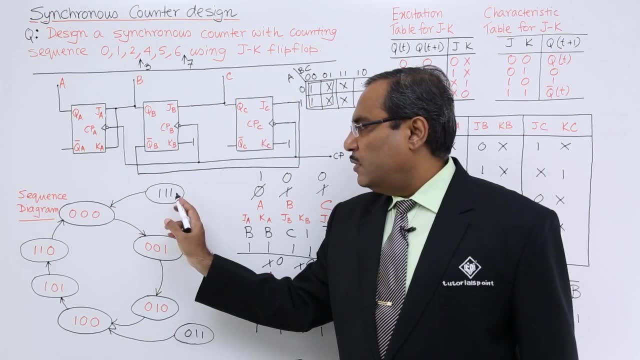 if I give the clock pulse next, my next state will be 0 0, 0.. So that is why I am putting here 1 1, 1 and from there. So this condition will be done from 1 1, 1 to 0 0, 0.. So now my sequence diagram has got completed. it is having all the eight. 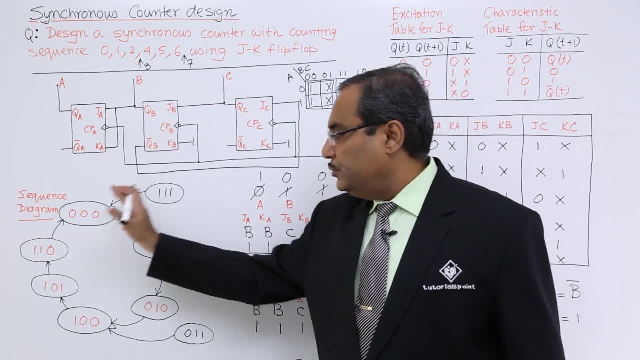 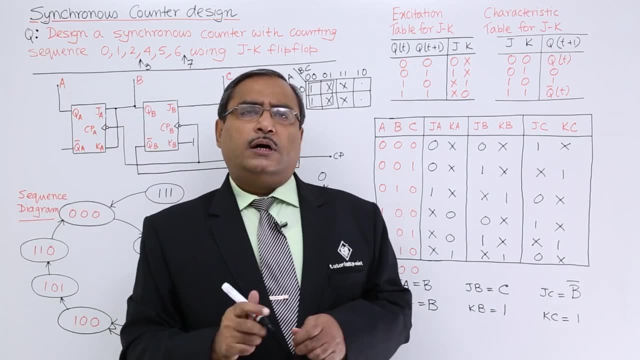 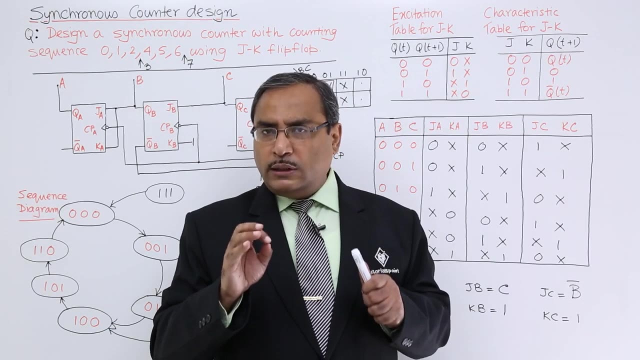 states starting from 0 to 7, and we have shown you that, how to complete this sequence diagram with this respective rough work. So I think now the circuit design for synchronous counter will not be a problem for you. I have given you all the tips that how to draw one synchronous counter here and at first you 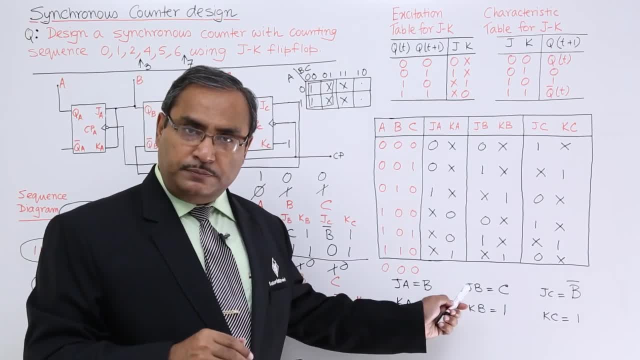 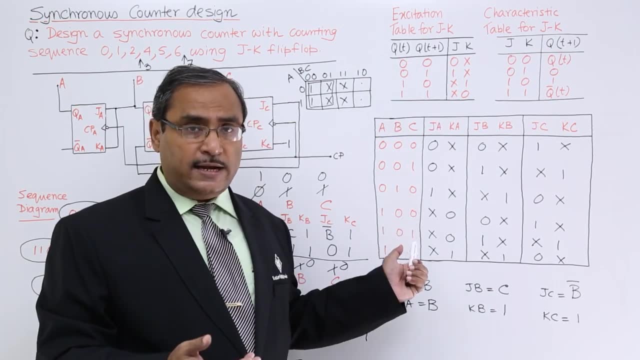 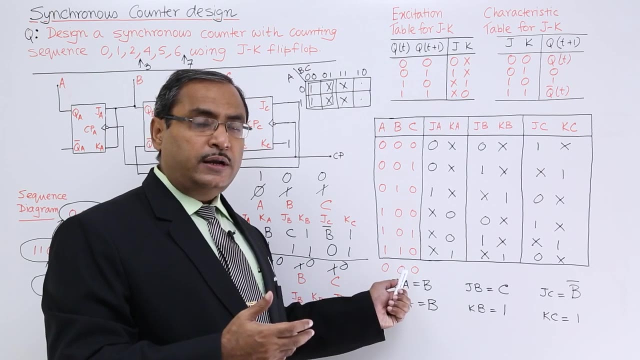 are supposed to go for this table construction, write the respective sequence, whether it is increasing or decreasing or random. some states might be missing, as we had here. So what about the sequence you require and also the first, ah, first term of the sequence, also written outside of the table, And then fill up them using your excitation table here. 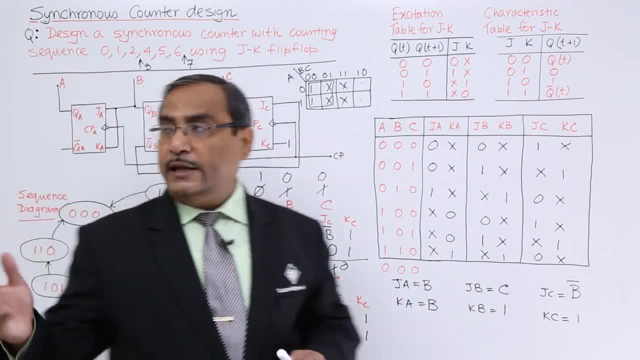 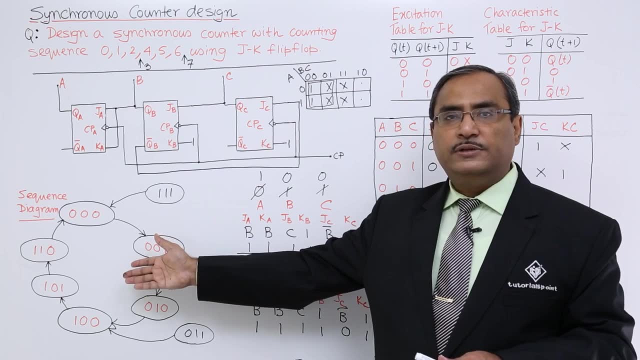 go for the summary, If you cannot get. go for the kernel map and then construct the circuit accordingly, complete with the connections, and then the circuit will be formed. Also, how to complete your sequence diagram, I have shown you, I think, now the synchronous counter. 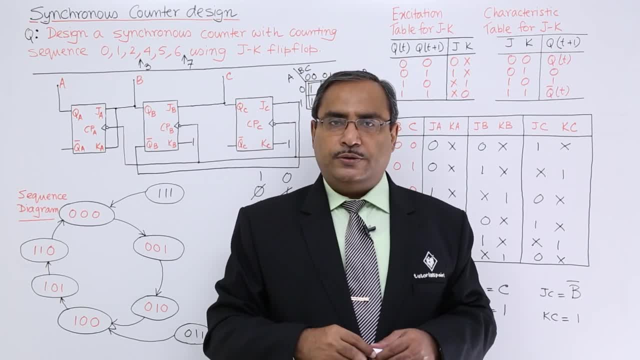 design will not be a problem for you. Thanks for watching this video. 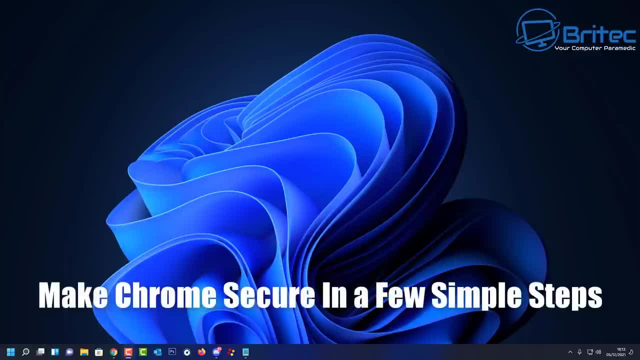 What you guys got another video here for you on making Chrome secure in a few simple steps. That's what we're going to be taking a look at today. So if you're using Google Chrome, then you want to make sure that you've got these settings in place to make sure that you're using the most. 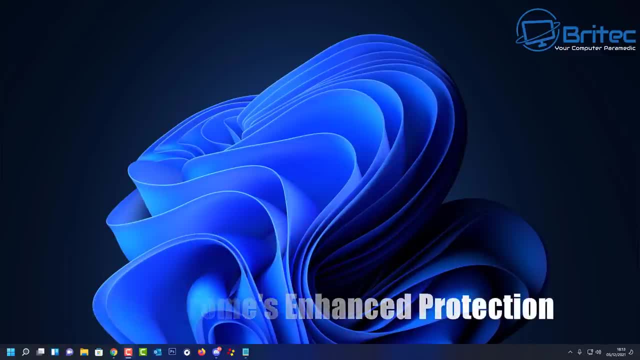 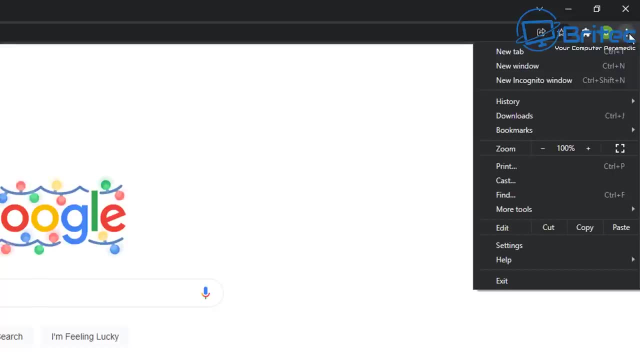 secure settings in Chrome. So enabling Chrome's enhance protection is the first thing that you want to do. So to do this, make sure you go up to the top right hand side here and click the three dots. We're going to come down to settings, inside settings. We're going to click on this one move.